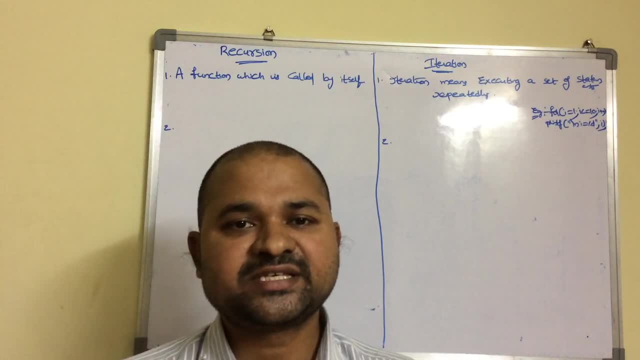 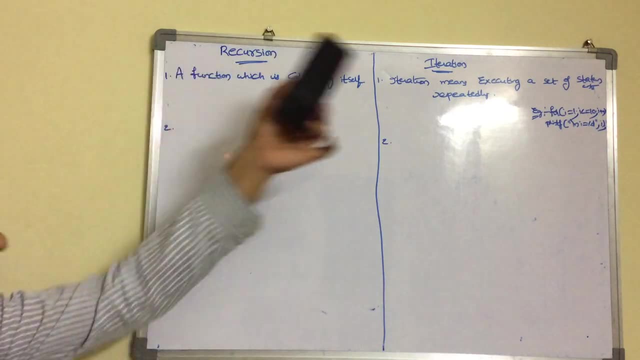 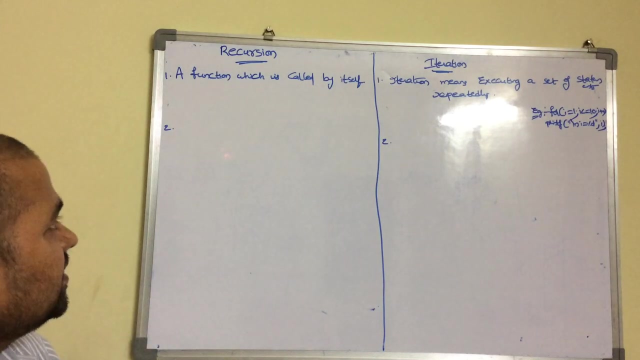 In this class we are going to discuss about the differences between recursion and iteration. So recursion, iteration. Here the first difference is the definition of recursion. A function which is called by itself is known as recursion. That means the calling function and the called. 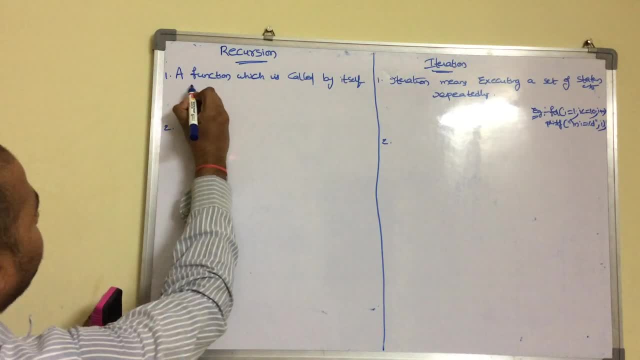 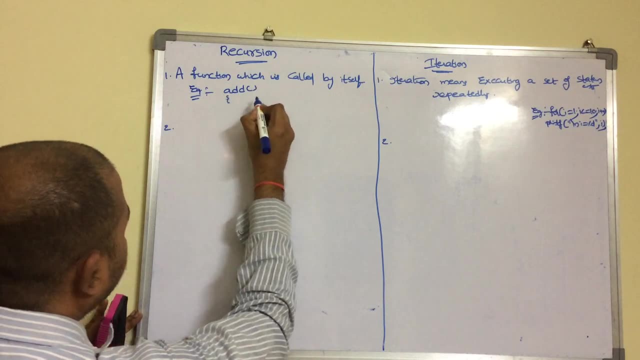 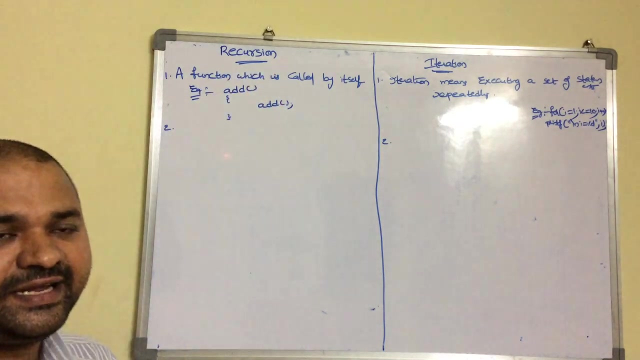 functions are same. Let's see an example Example. So we are defining a function called add function. In the add function we are calling the add function. So this is an example for recursion. Why? Because here this add function is calling function. 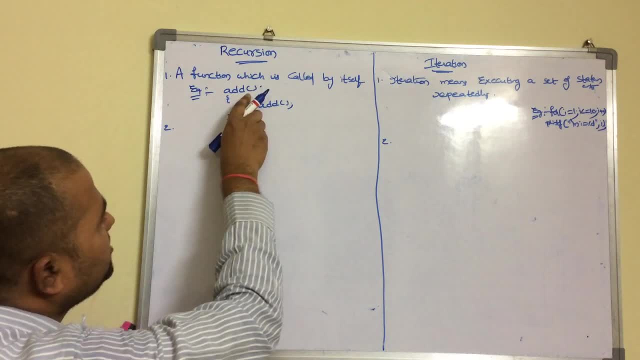 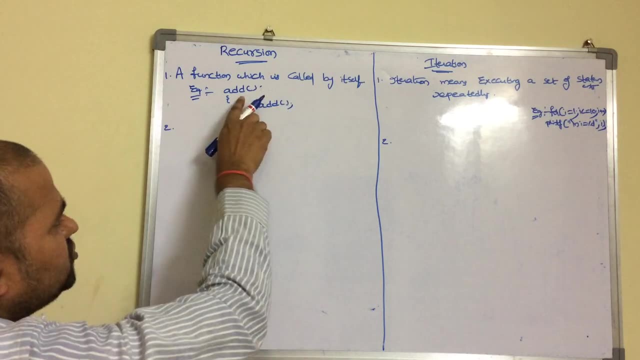 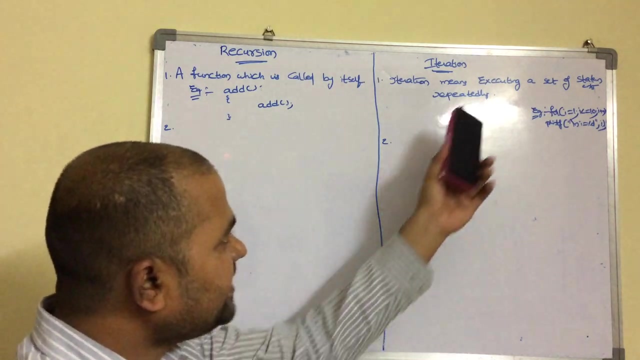 So why? Because this add function is calling function. In the add function we are defining the add function, So this add function is called function. So both calling and called functions are same. So that's why it is an example for recursion: Various iteration means. 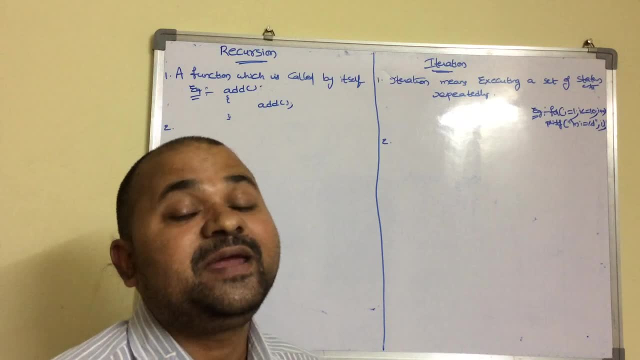 executing a set of statements repeatedly. as long as the condition is true, Iterative control statements are nothing but a set of statements. So this is a set of statements. So this is a set of looping control statements. We have three looping control statements. First one: 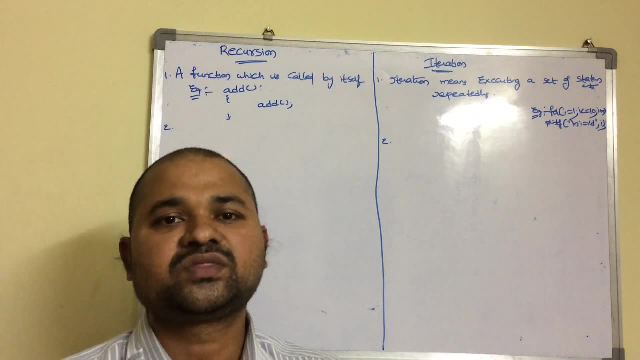 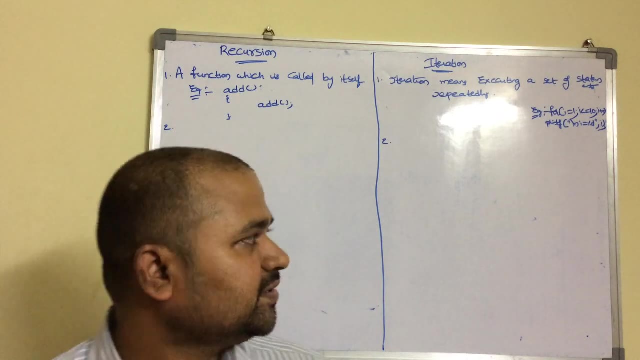 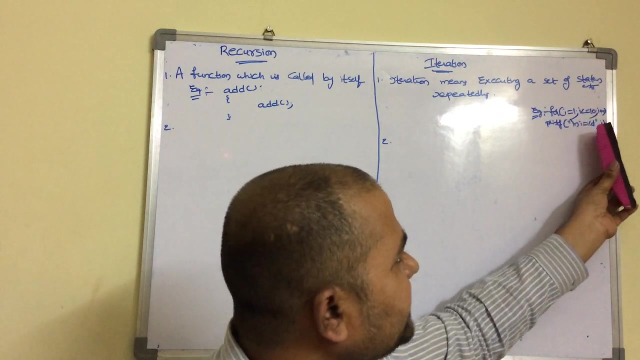 for loop. Second one while loop. Third one: do while loop. Here let us take an example of printing the numbers from 1 to 10.. For i is equal to 1, i less than or equal to 10, i plus plus, Print up slash and i is equal to percentage d comma i. So in the first iteration 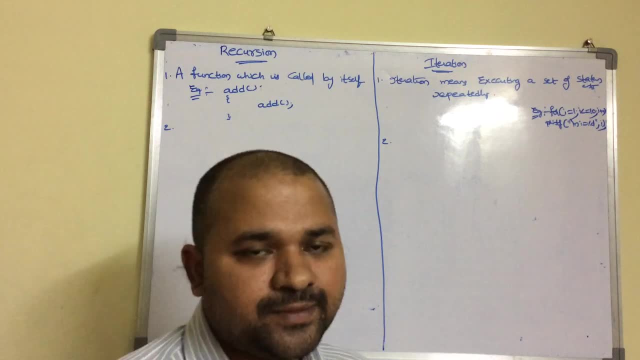 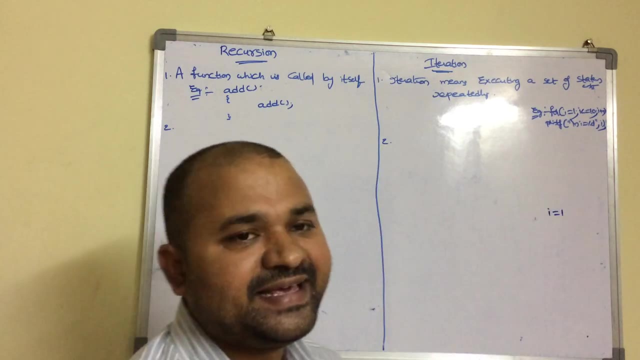 i is equal to 1.. 1 less than or equal to 10. Condition is true. So the output here is i is equal to 1.. So in the first iteration i is equal to 1 will be printed. Next i becomes 2.. 2 is less than or equal to 10. Condition: 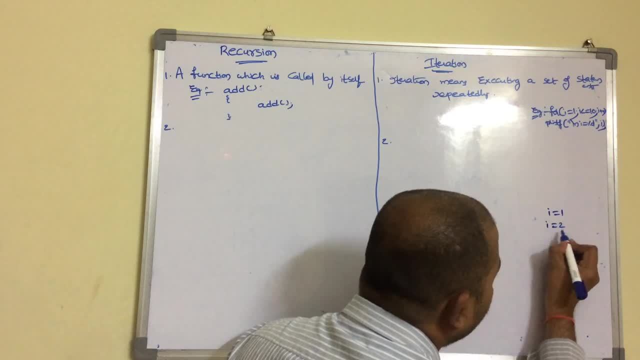 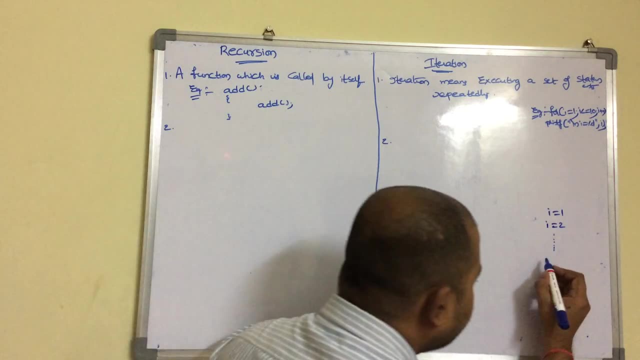 is true. So in the second iteration i is equal to 2 will be printed. Likewise, the for loop will be executed for 10 iterations. So in the last iteration i is equal to 10 will be printed. Next i becomes 11.. 11 less than or equal to 10.. so it is his Then i. 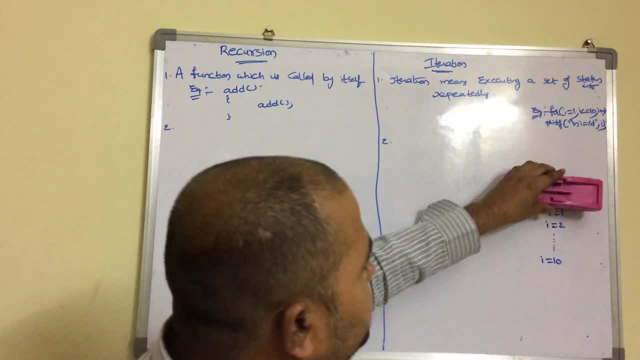 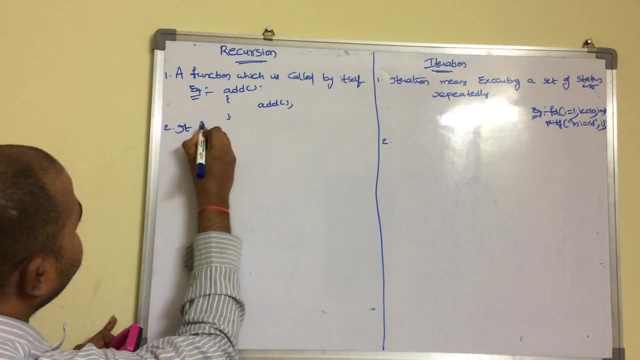 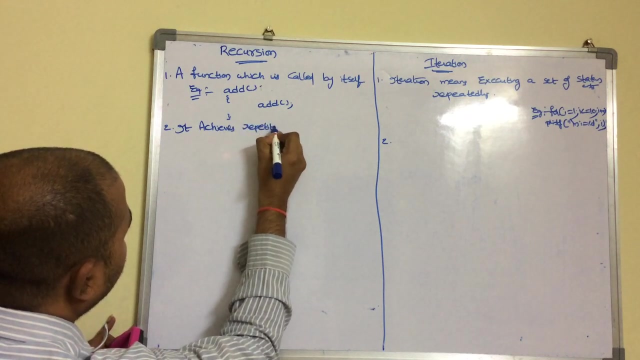 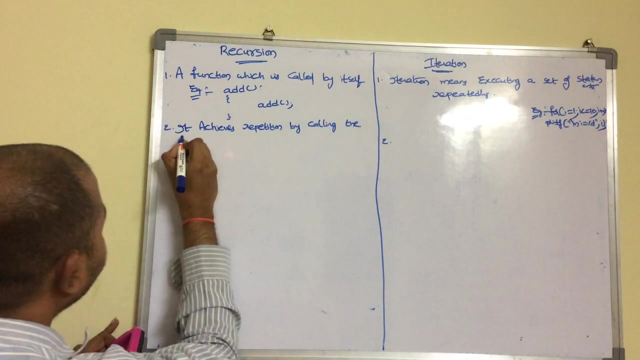 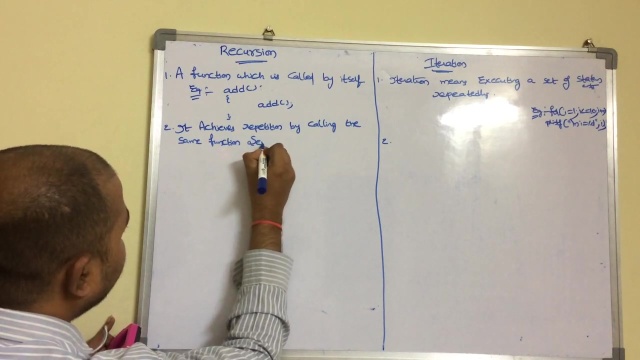 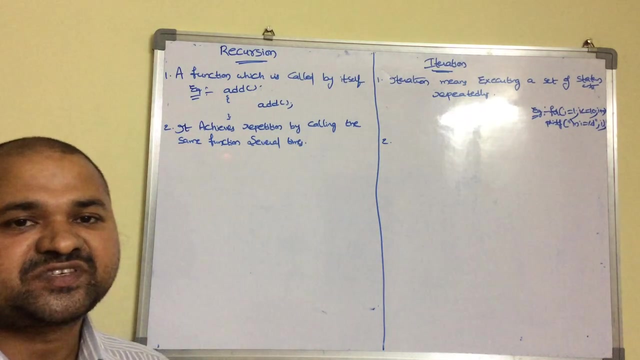 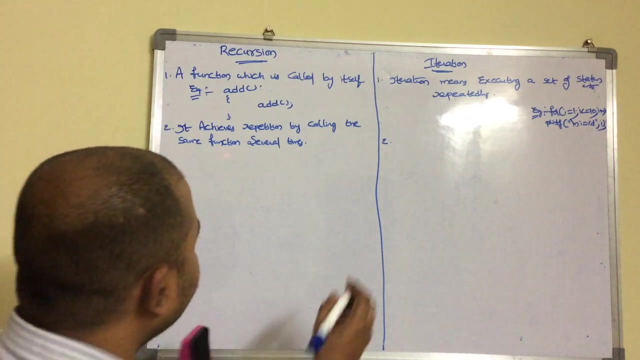 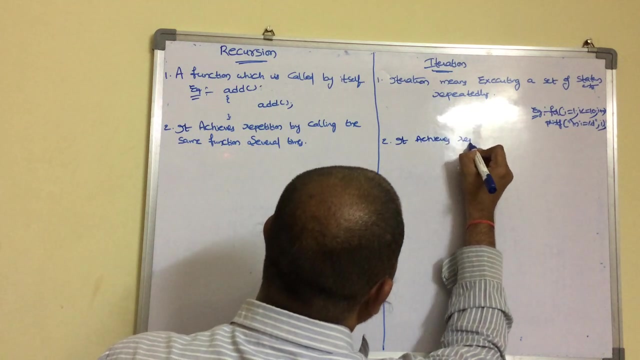 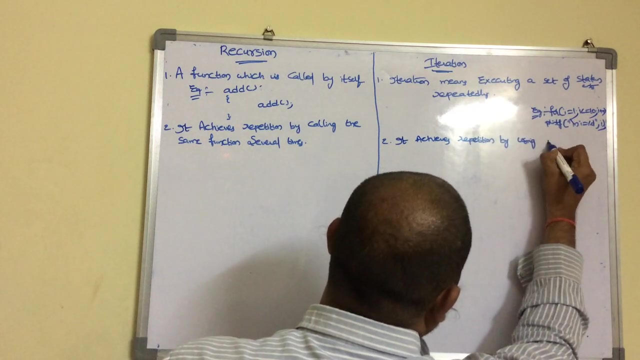 becomes宅 14. Condition is false. So control comes out from the faculty. Now let us see the second difference It achieves in recursion. we achieves repetition by calling the same function, the same function, several times, Many times. So in recursion we achieves repetition by calling the same function many times Various. in iteration we achieves repetition. It achieves repetition by using iterative function. 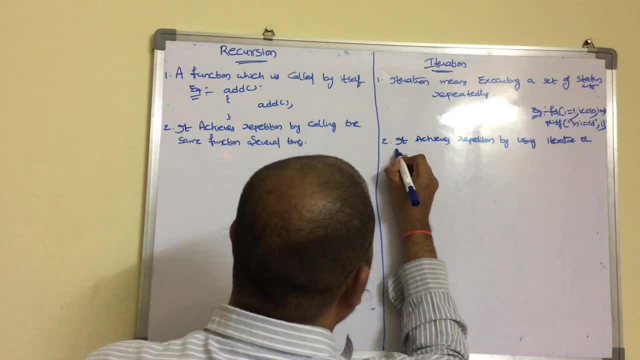 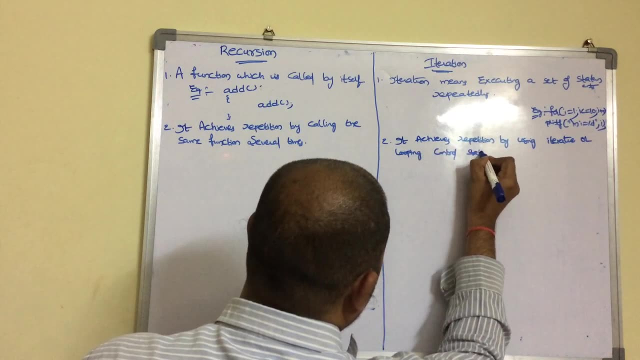 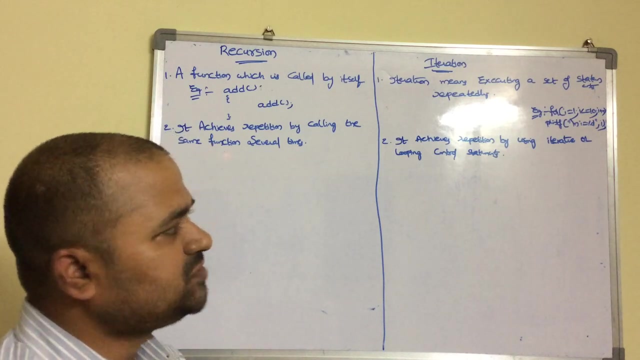 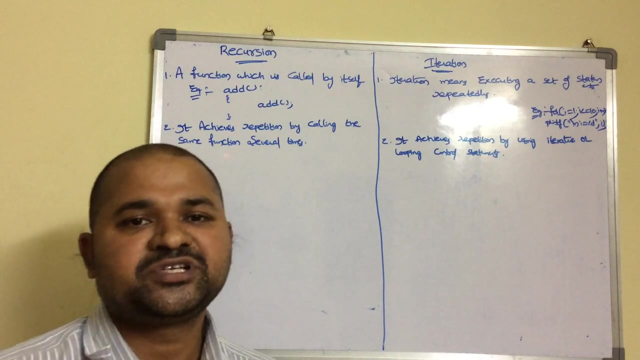 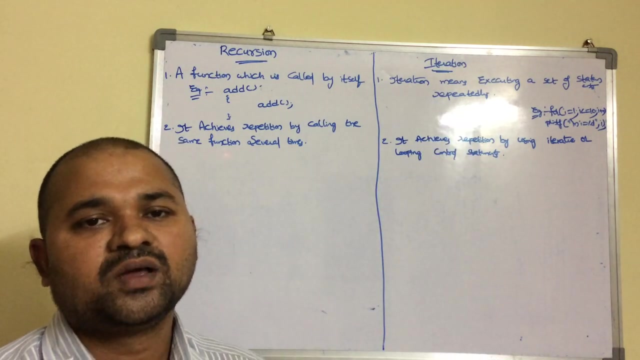 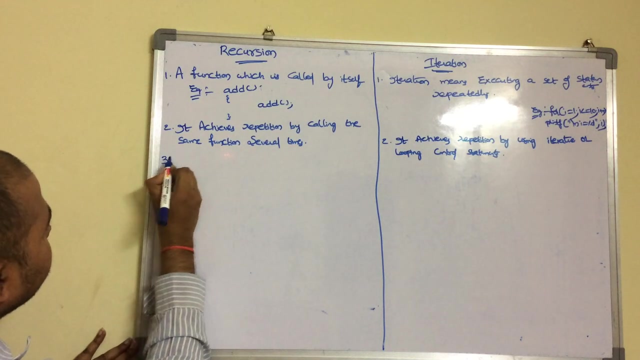 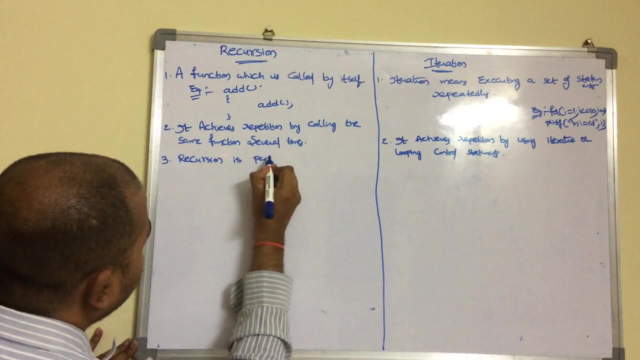 So iterative or iterative or looping control statements. So we achieve repetition by using either iterative or looping control statements. So already I said that iterative control statements are also known as looping control statements. So the best examples for iterative or looping control statements are for loop while loop and the third one is do while loop. And the third difference is recursion is performed on a function. 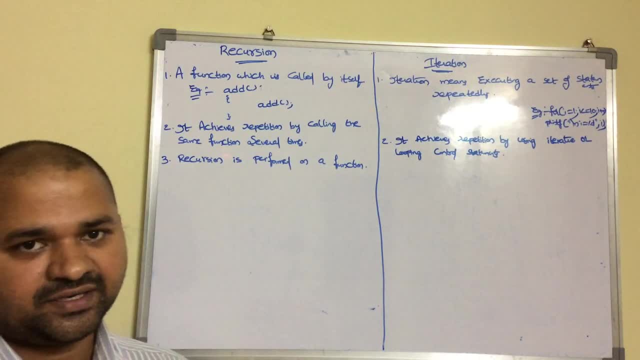 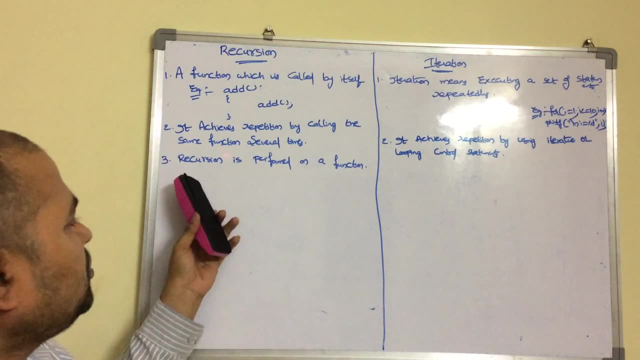 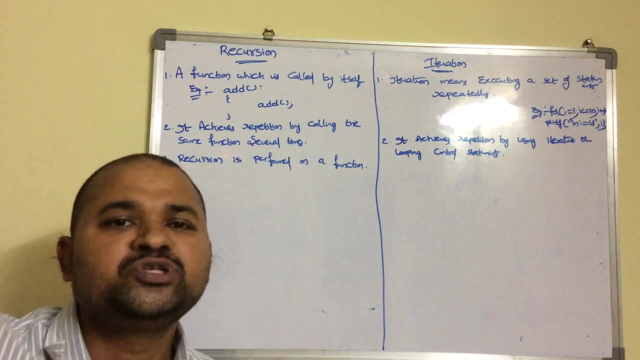 So if we want to implement recursion, then we must use functions. Without defining the functions, it is not possible to implement recursion. So that is the third point. We can perform recursion only on some user defined functions. The functions which are defined by the user are known as user defined functions. 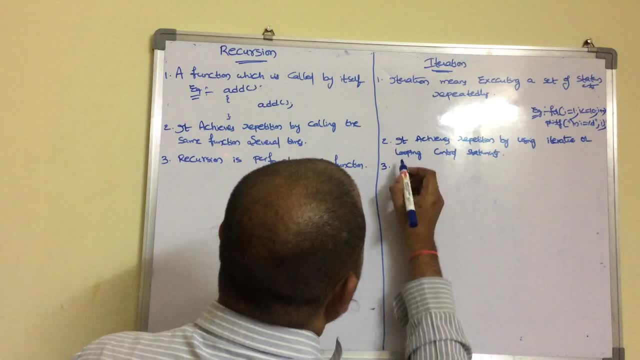 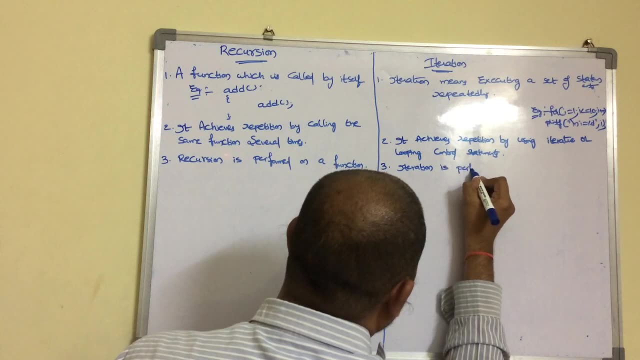 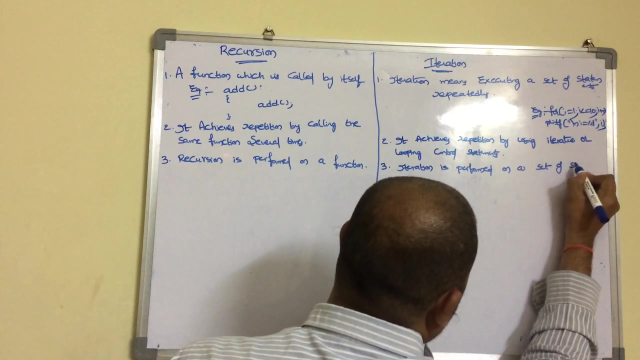 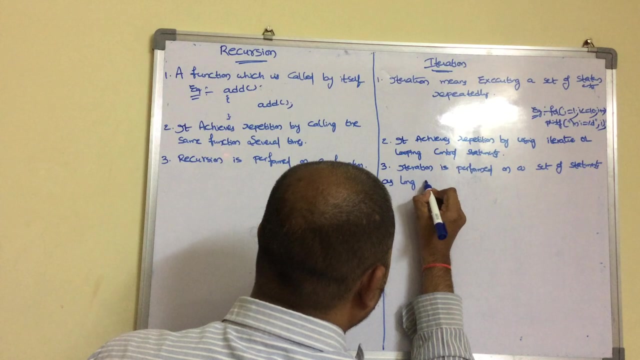 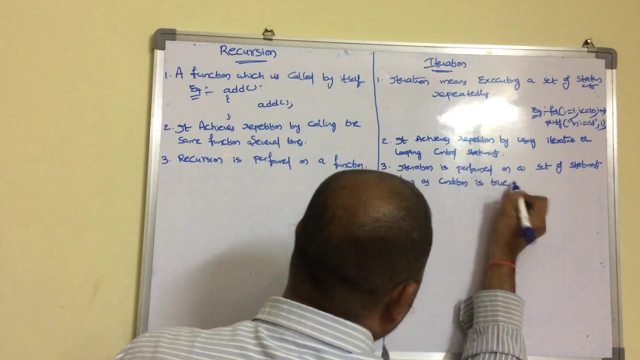 And here the third point is: iteration is performed on A set of statements. So set means collection on a set of statements, as long as condition is true. So we can perform iteration on a set of statements, A collection of statements, As long as condition is true. 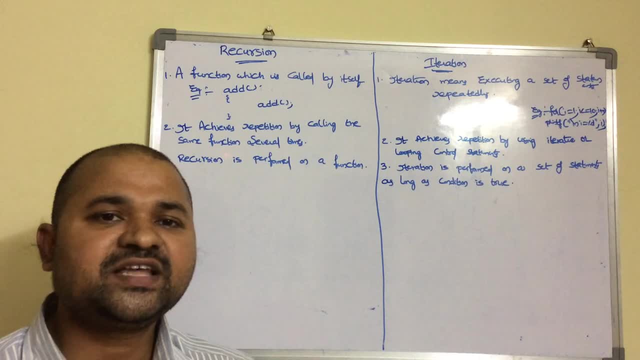 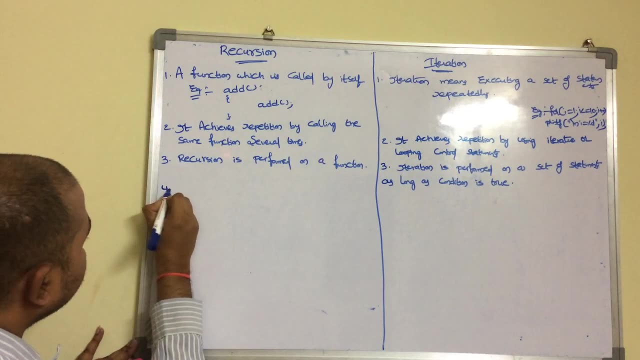 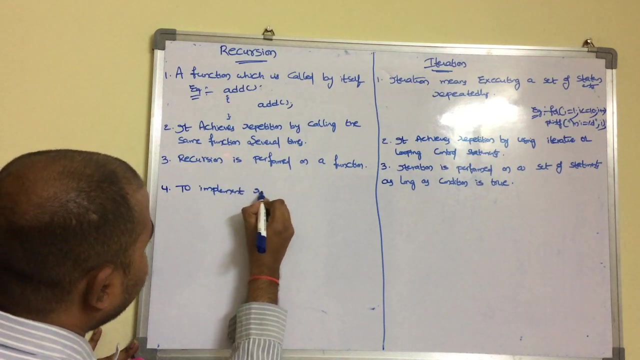 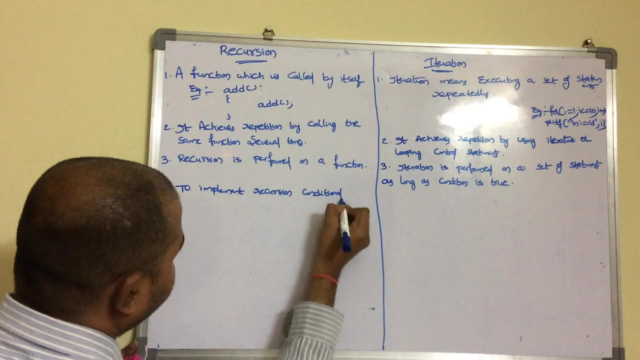 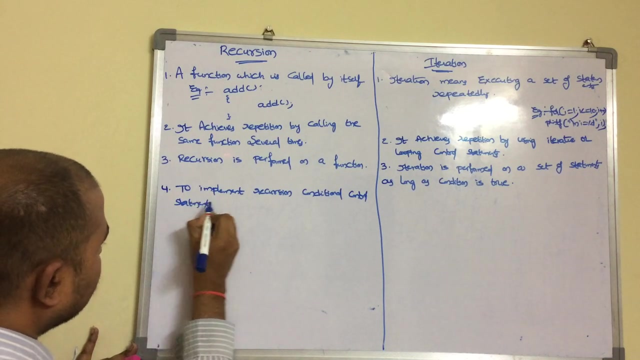 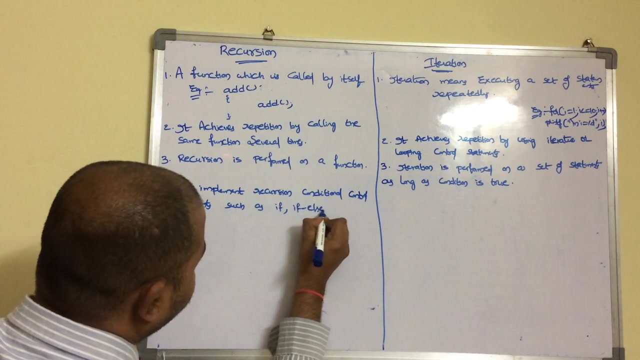 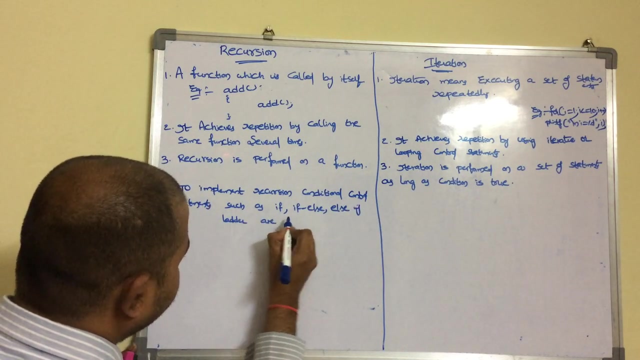 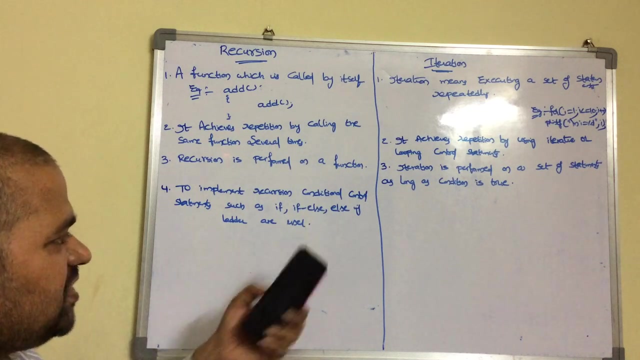 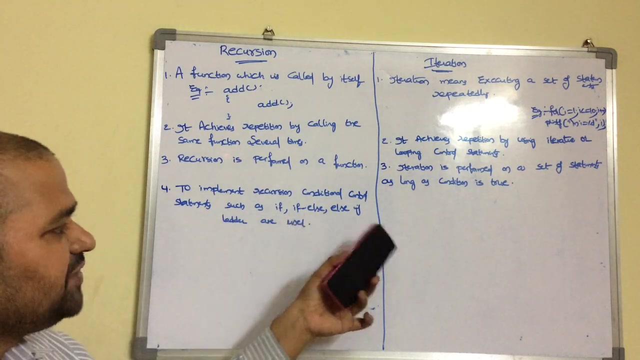 So whenever the condition becomes false, Then the control comes out from the loop. and here the next point is to implement recursion. to implement recursion, conditional control statements, conditional control statements such as if comma, if else, comma, else, if ladder- are used. So if you want to implement any recursive function, then we must use conditional control statements or selection control statements such as if, if else and else, if ladder, If there is only one condition in the function. 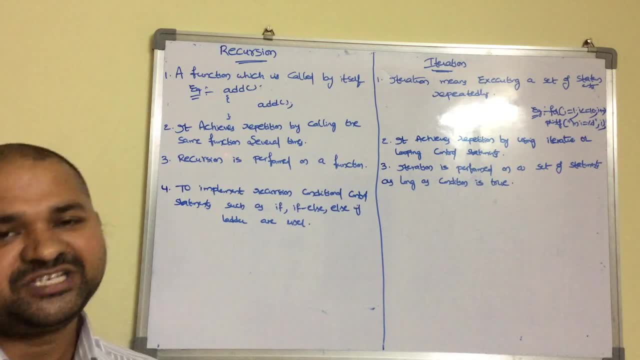 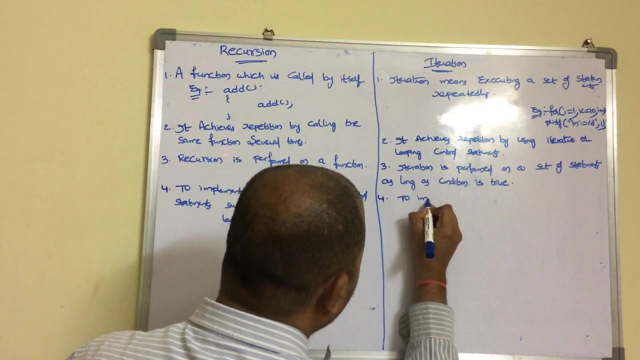 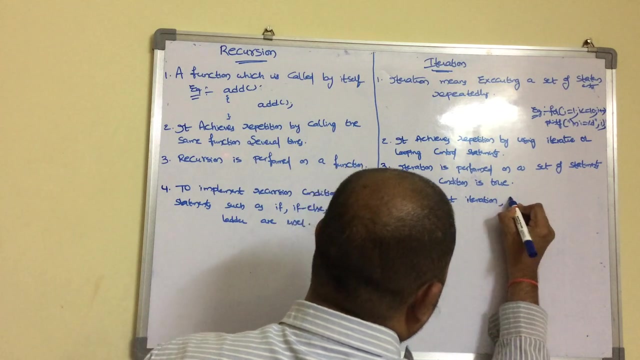 then we use. if If there are two conditions, then we use. if else, If there are more than two conditions in the recursive function, then we go for else. if ladder Various here. the fourth point is to implement iteration, iterative control statements. Iterative control statements means loop. 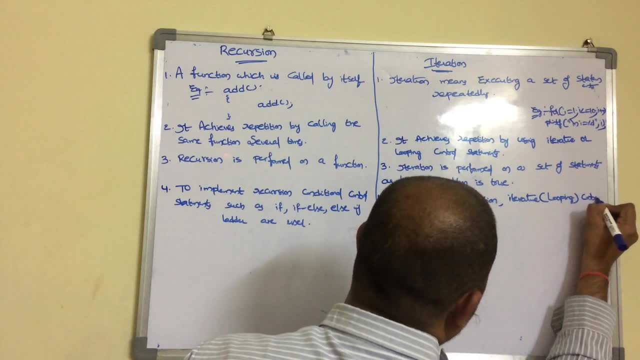 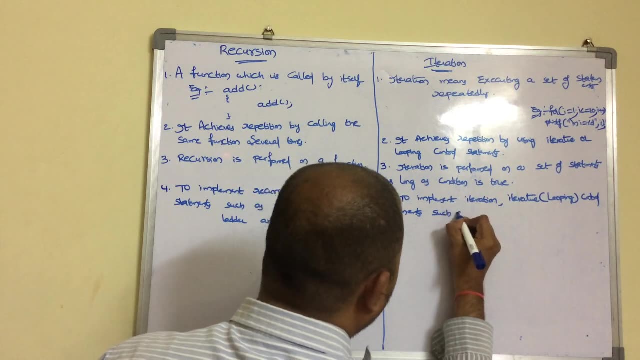 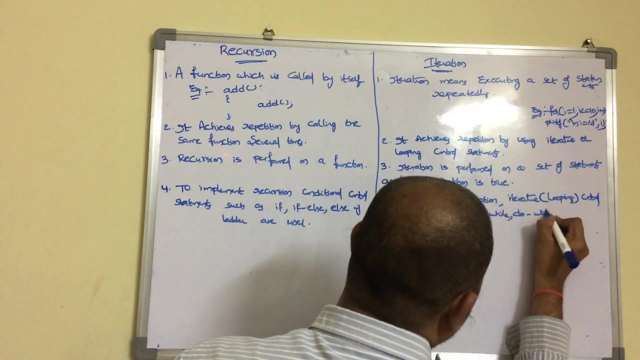 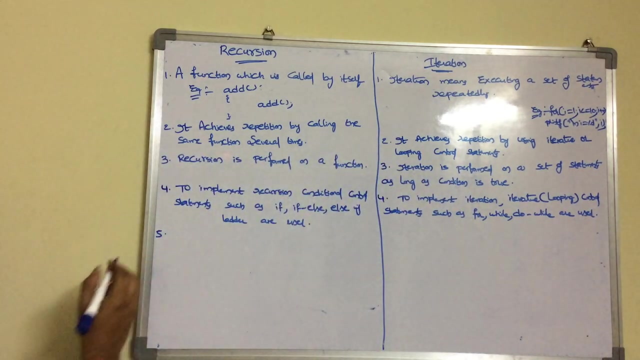 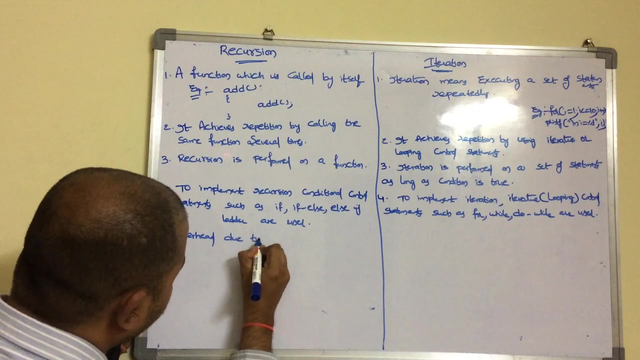 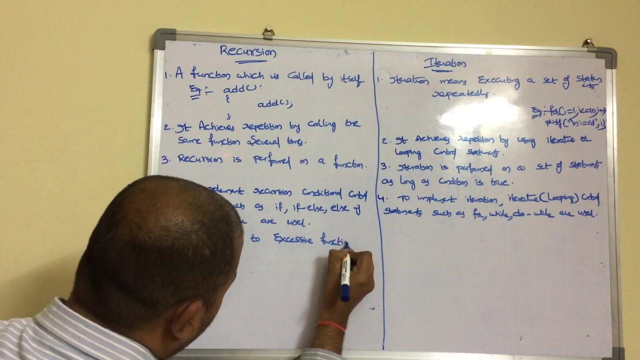 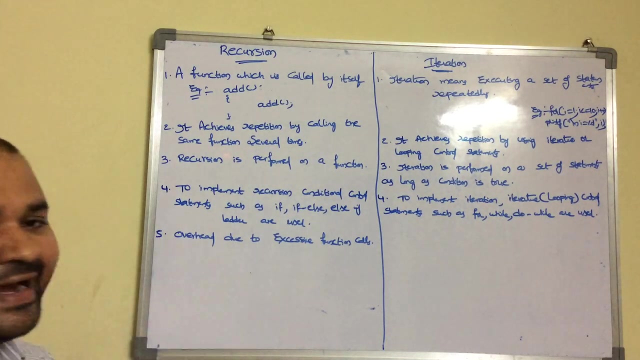 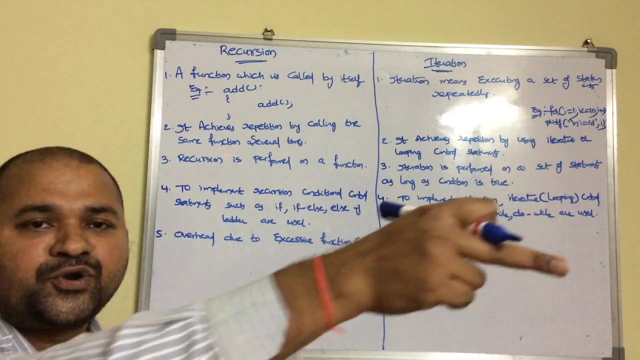 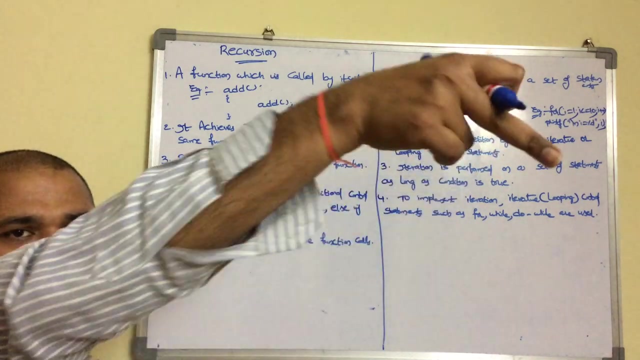 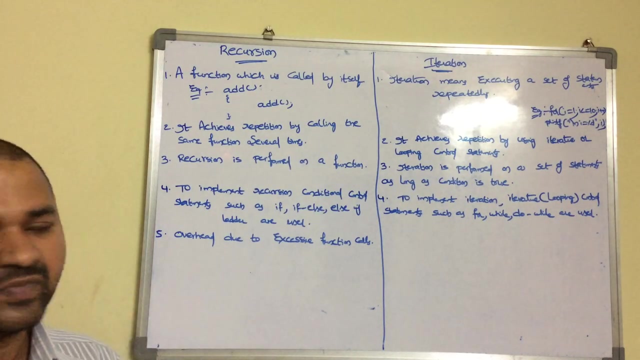 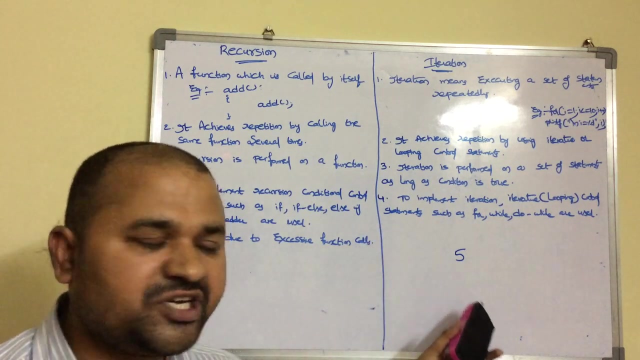 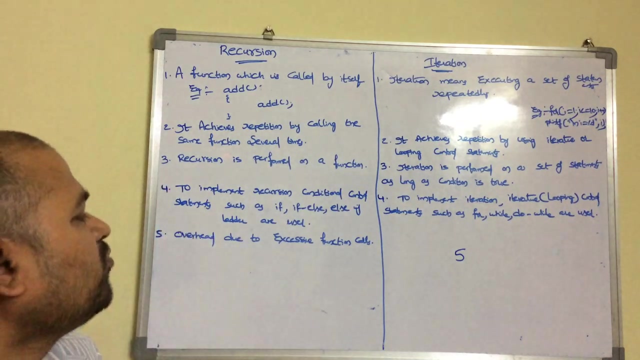 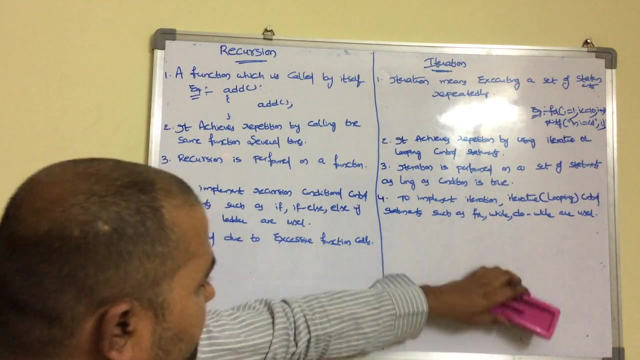 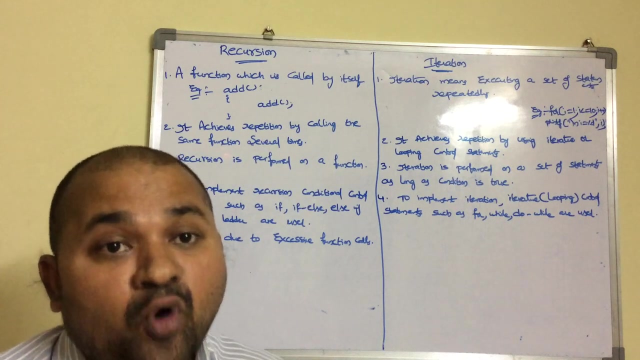 looping control statements, Iterative control statements such as: So what are the iterative control statements For comma while? comma do while are used? And the next point is overhead. overhead due early due to excessive function calls Various. if you take iteration, we are calling the function only one time, so there is no overhead on the compiler. 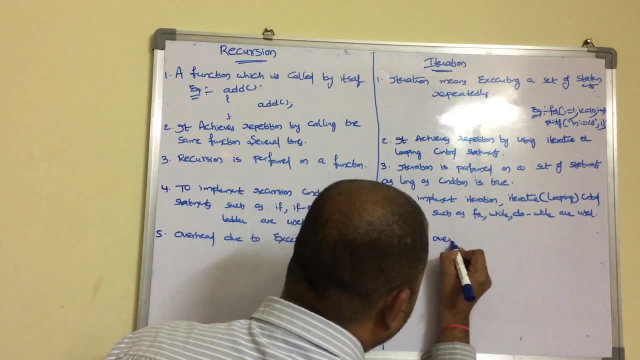 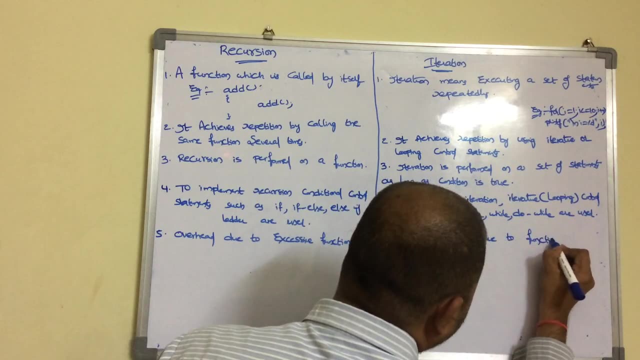 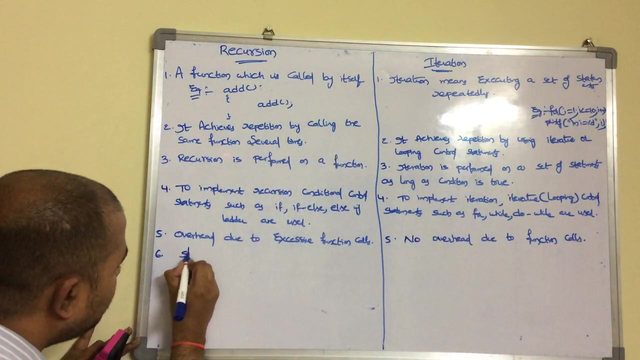 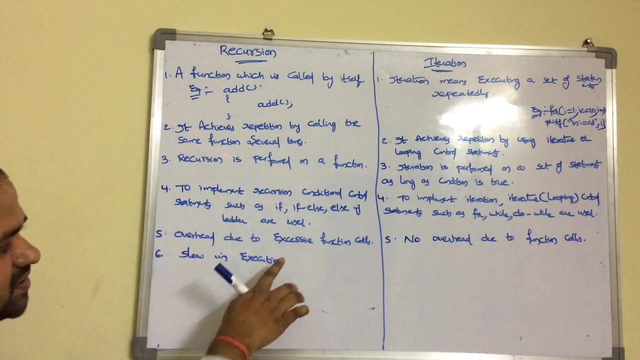 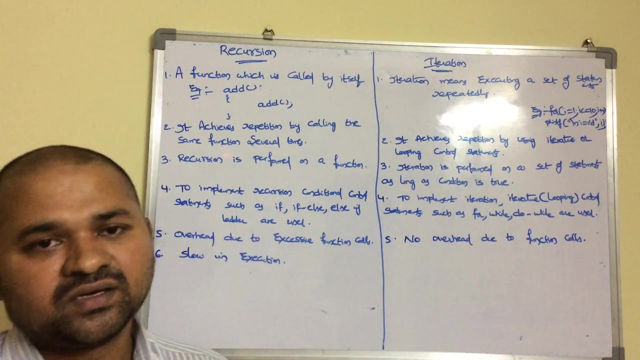 What is the point? No overhead due to function calls. Why? Because there is only one function call. And the next point is: recursive programs are slowly in execution. why? because we are calling the same function several times, so there is a lot of overhead on the compiler as. 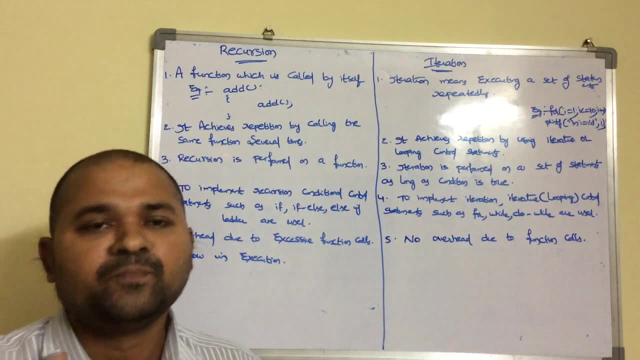 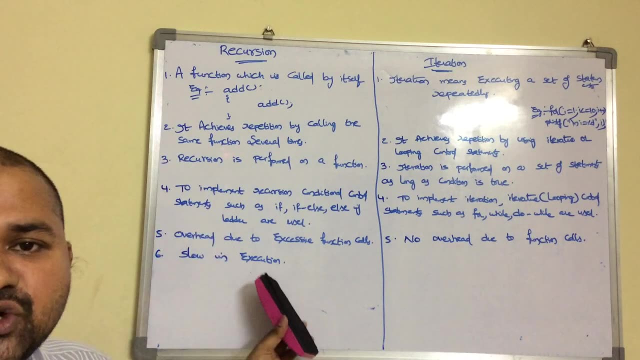 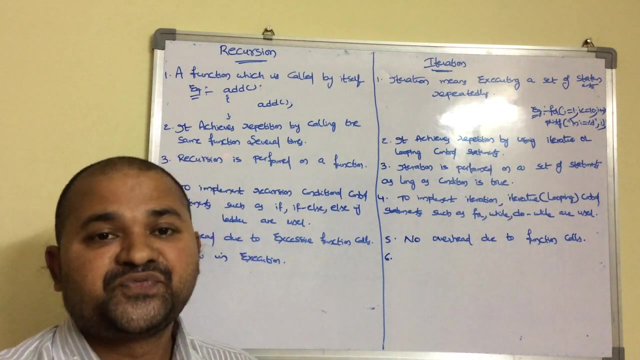 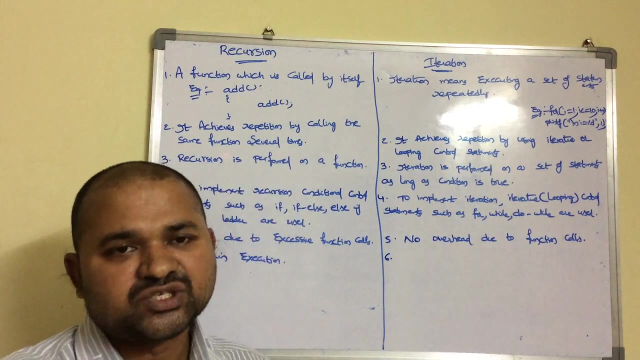 well as so a recursive programs takes more time in order to execute the program, so we can say that recursive programs are slow in execution, whereas iterative programs are faster in execution. why? because we are calling the function only once, so there is no overhead, so iterative programs are